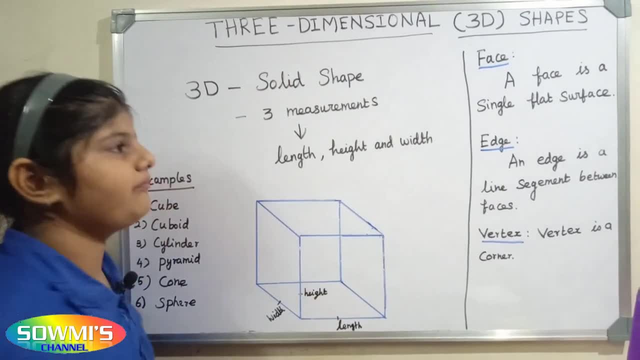 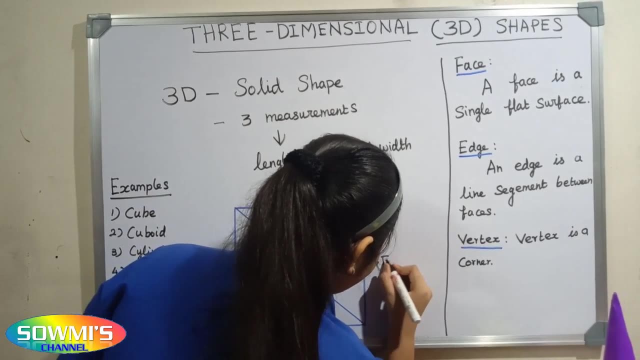 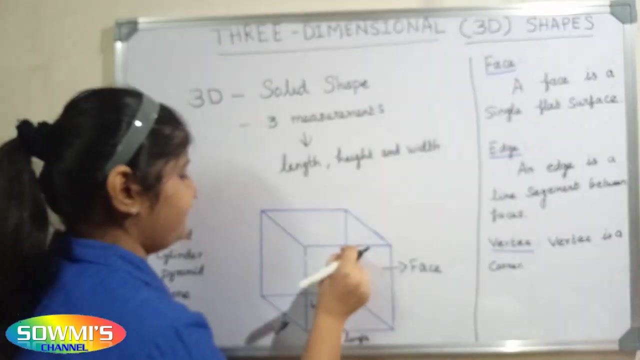 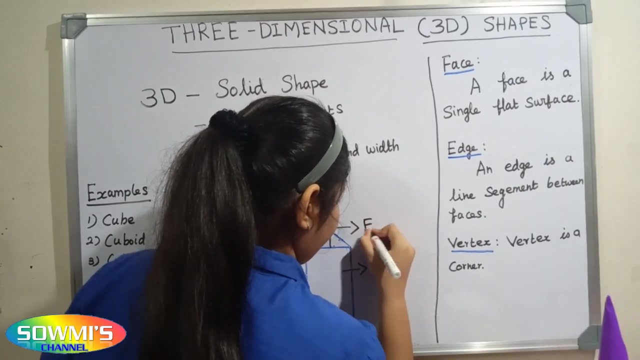 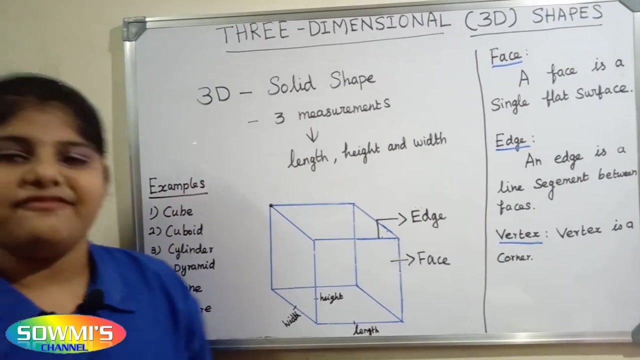 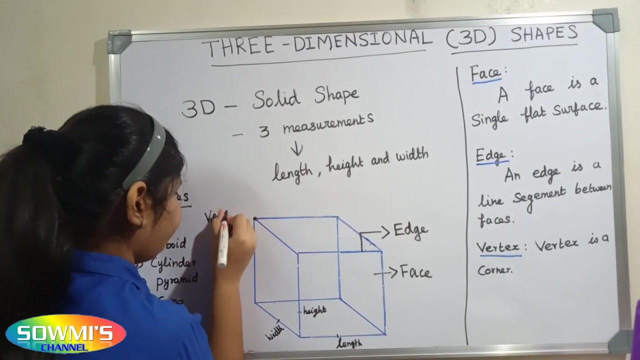 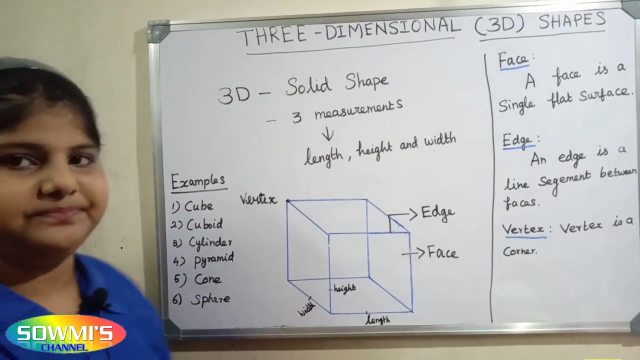 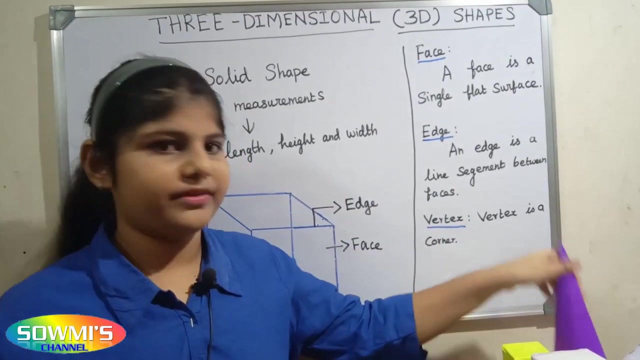 width. This is the face of a cube. A face is a single flat surface. This is the edge of a cube. An edge is a line segment between two faces. This is the vertex. This is the vertex. Vertex is a corner of a cube. Examples for 3D shapes are cube, cuboid, cone, cylinder. 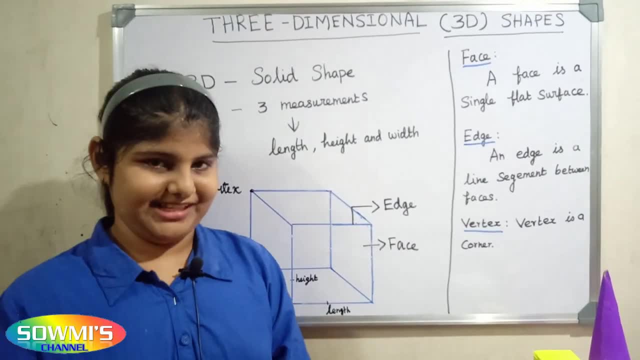 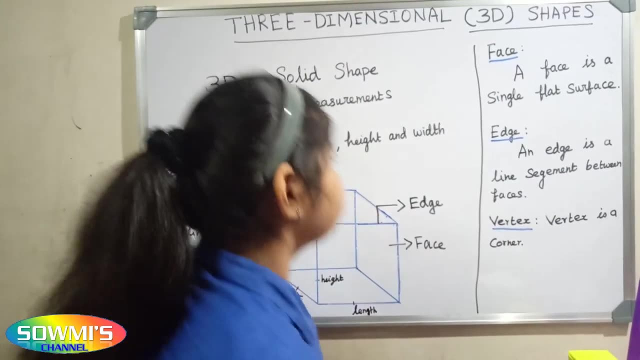 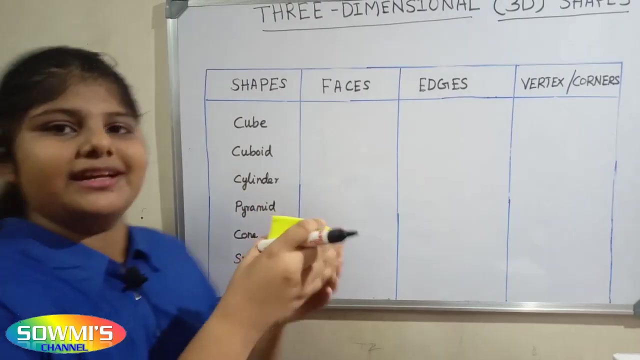 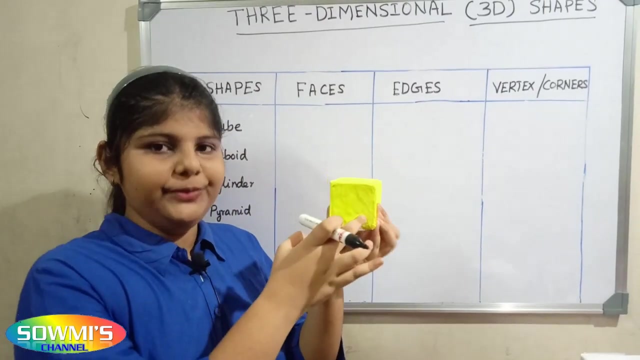 etc. Next we will see how to count face edge and vertex of 3D shapes. First we will take cube. This is a cube. First we will count the faces in a cube: 1,, 2,, 3,, 4,, 5, 6.. There 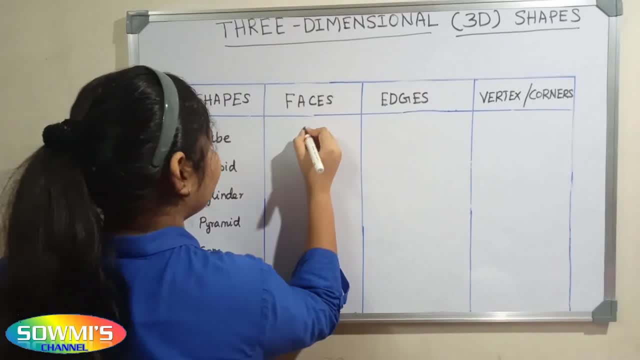 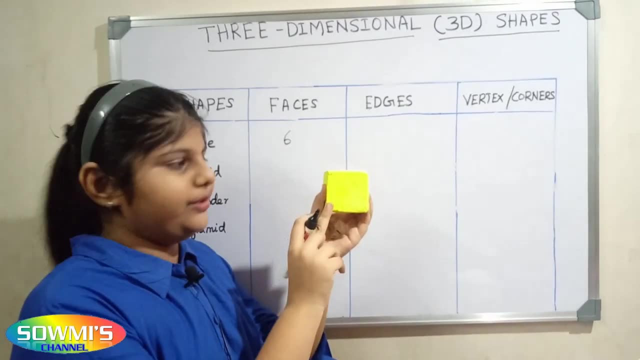 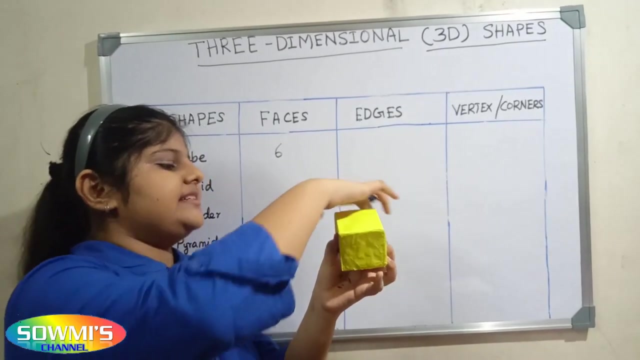 are 6 faces in a cube. Next we will count the edges in a cube: 1,, 2,, 3,, 4,, 5,, 6,, 7,, 8,, 9,, 10,, 11,, 12.. 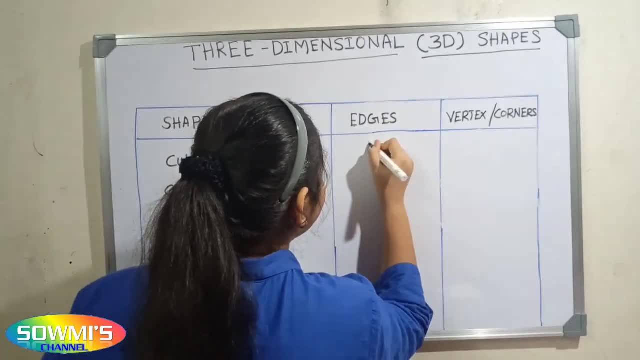 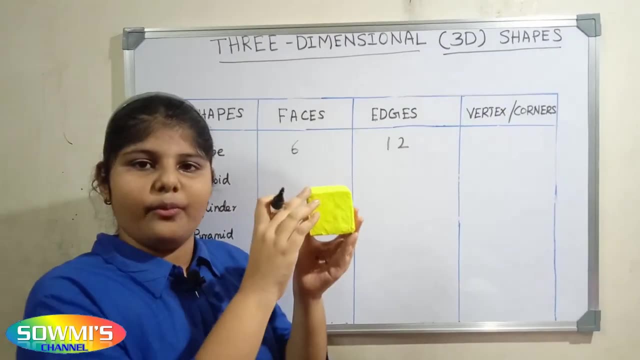 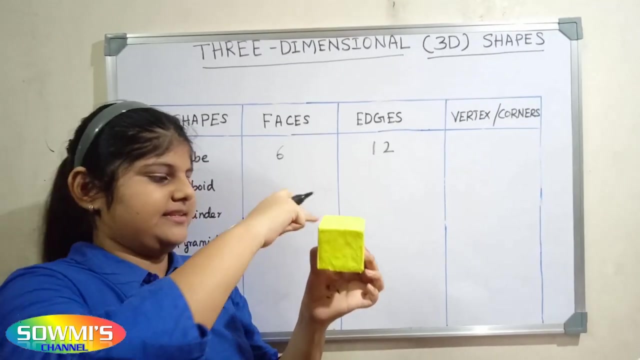 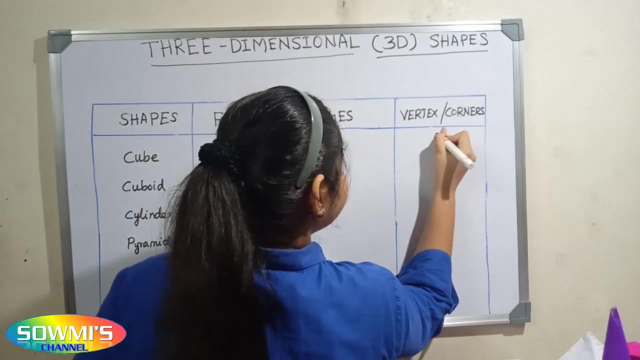 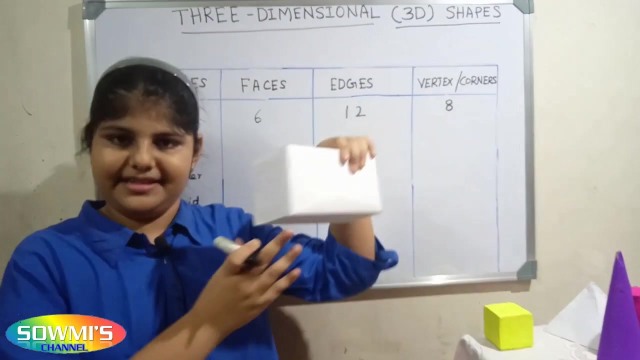 There are 12 edges in a cube. the corners in a cube 1,, 2,, 3,, 4,, 5,, 6,, 7, 8.. There are 8 corners in a cube. Next we will take cuboid. This is the cuboid First. we will count the faces in a cuboid: 1,, 2,. 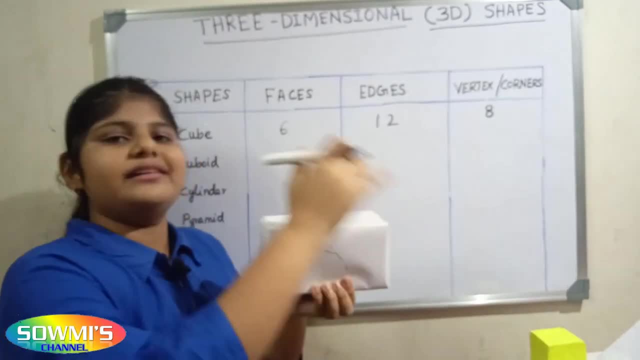 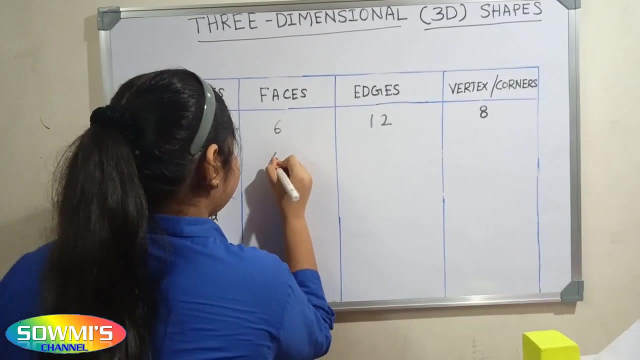 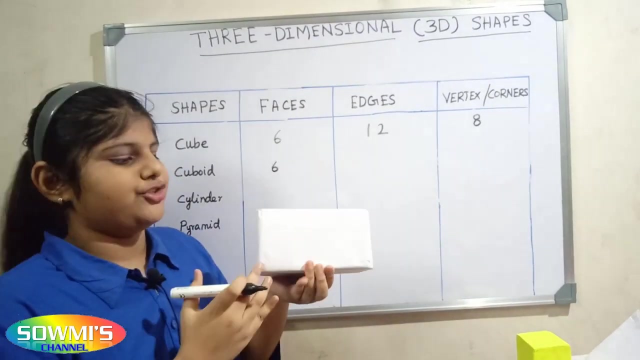 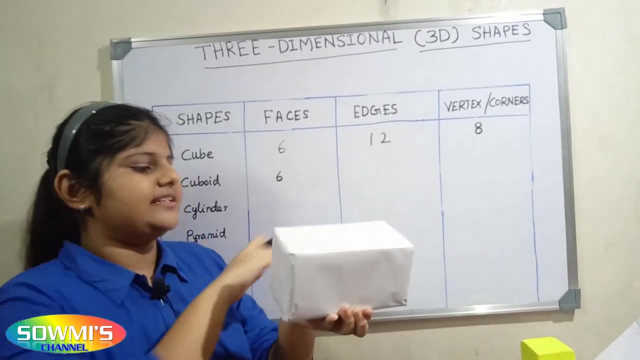 3,, 4,, 5, 6.. There are 6 faces in a cuboid. Next we will count the edges in a cuboid: 1,, 2,, 3,, 4,, 5,, 6,, 7,, 8,, 9,, 10,, 11,, 12.. There are 12 edges in a cuboid. Next we will count. 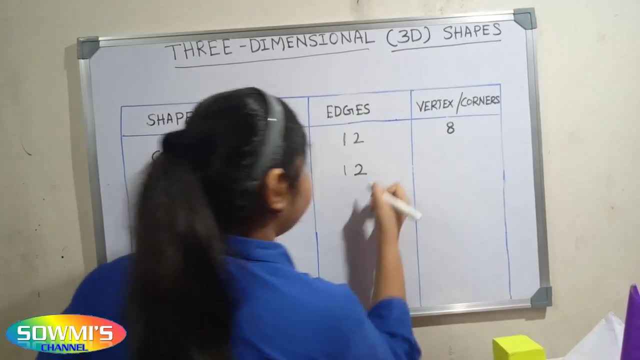 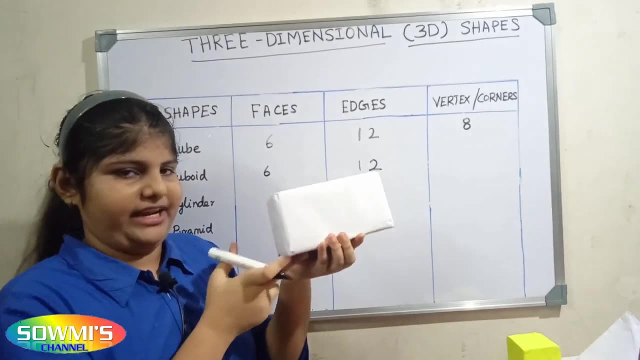 the corners in a cuboid: 1,, 2,, 3,, 4,, 5,, 6,, 7, 8.. There are 8 corners in a cuboid: 1,, 2,, 3,, 4,, 5,, 6,, 7,, 8.. There are 8 corners. 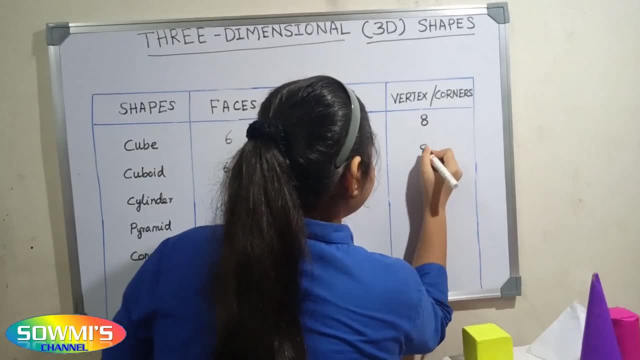 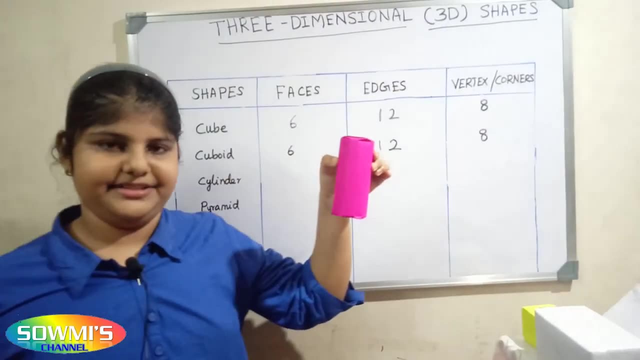 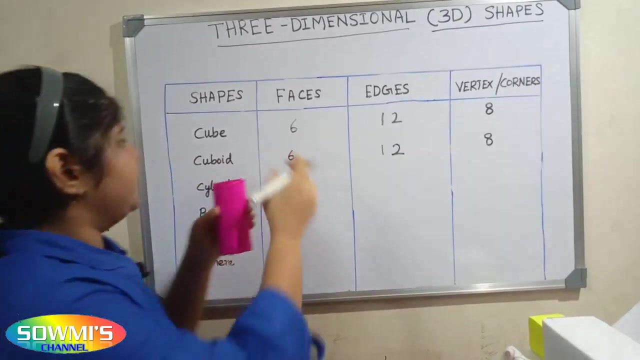 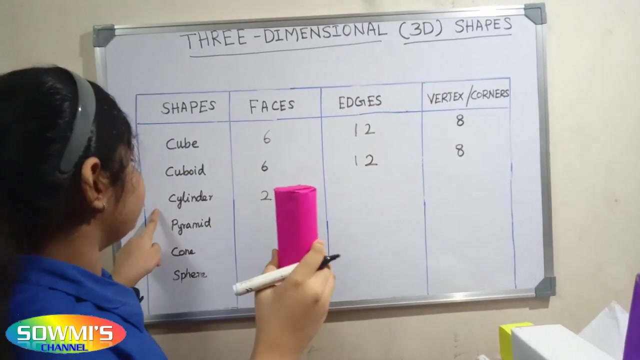 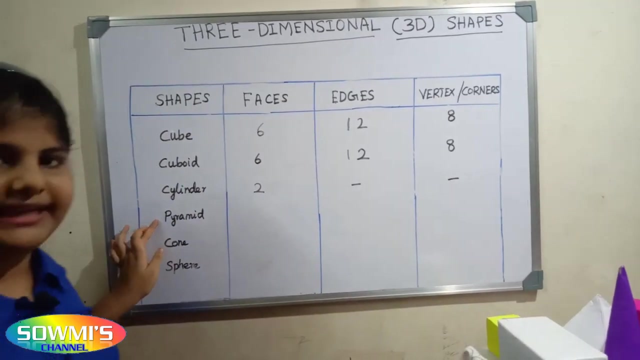 in a cuboid. Next we will take cylinder. This is the cylinder. first we will count the faces in a cylinder. there are one, two, two faces in a cylinder. there are no edges and corners in a cylinder. next we will take pyramid. this is the pyramid. first we will count the faces of the pyramid. 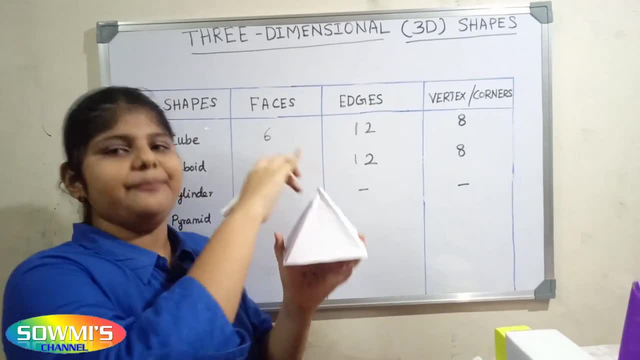 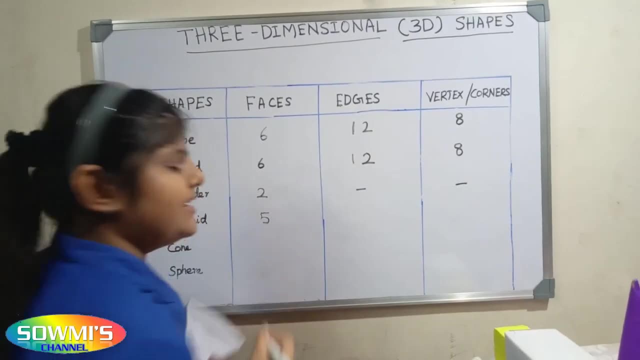 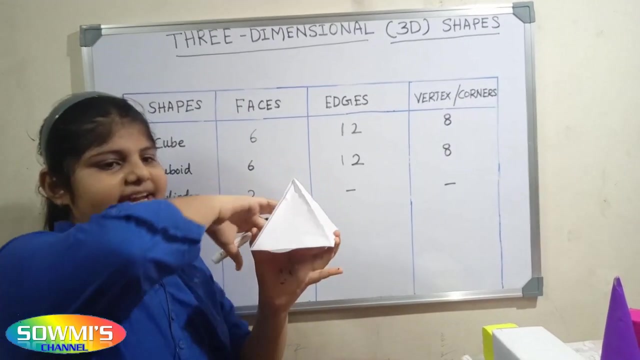 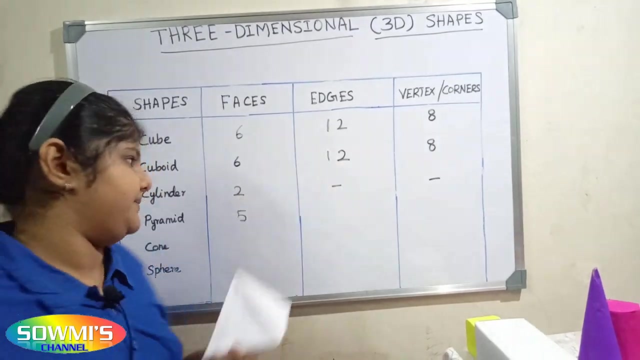 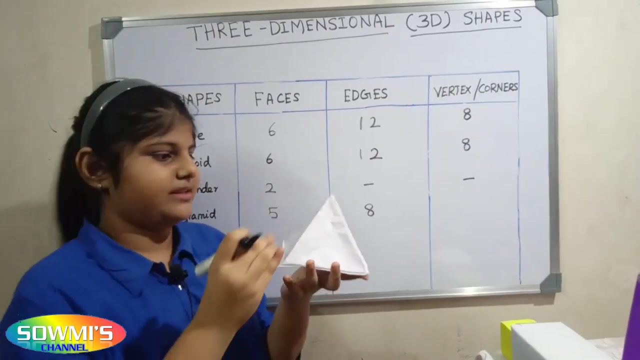 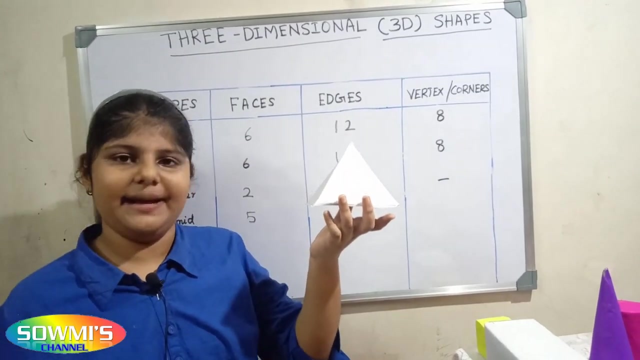 one, two, three, four, five. there are five phases in a pyramid. next we will count the edges in a pyramid: one, two, three, four, five, six, seven, eight. there are eight edges in a pyramid. next we will count the corners in a pyramid pyramid. One, two, three, four, five. There are five corners in a pyramid. Next we 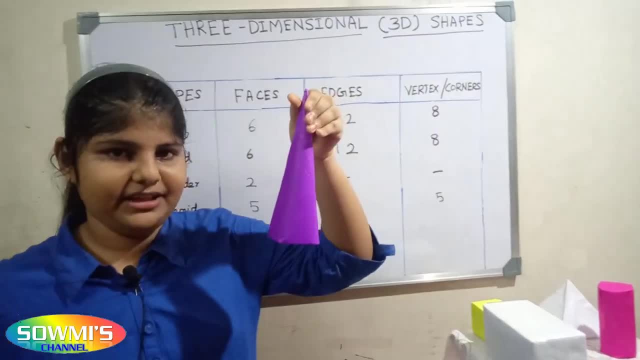 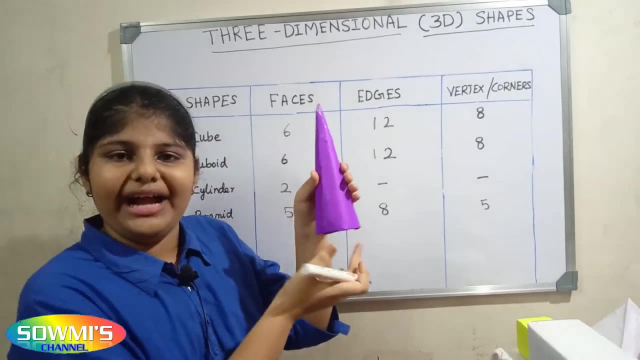 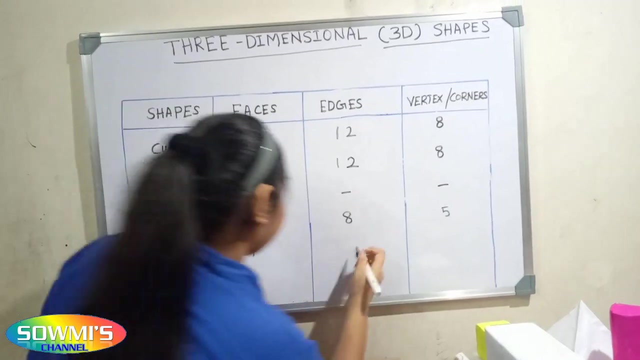 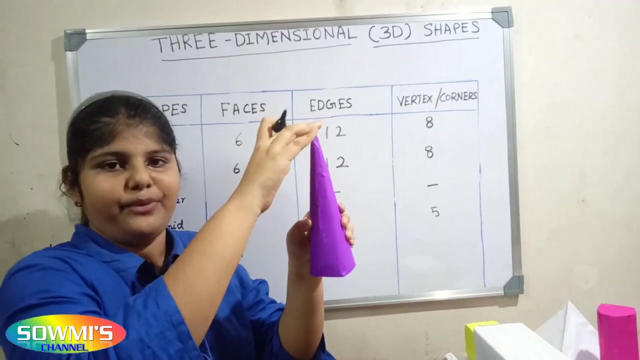 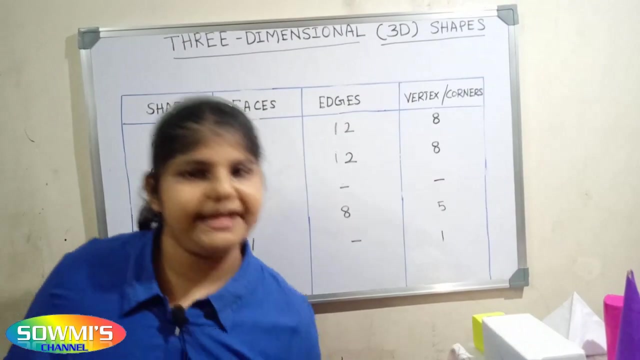 will take cone. This is the cone. First, we will count the faces in a cone. There is only one face in a cone. There are no edges in a cone. Next, we will find corners in a cone. There is only one corner in a cone. Next, we will take spear. This is the spear.